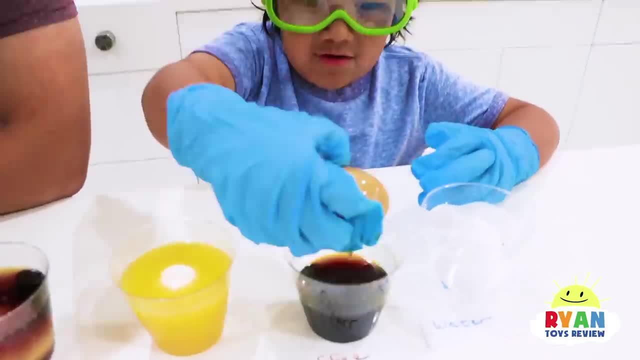 Next, let's look at the egg in coffee. This is my teeth. Awww, I thought I'd brush my teeth. Look at this. What happened to the egg Ryan? It sprung. It changed the color. Look at it. 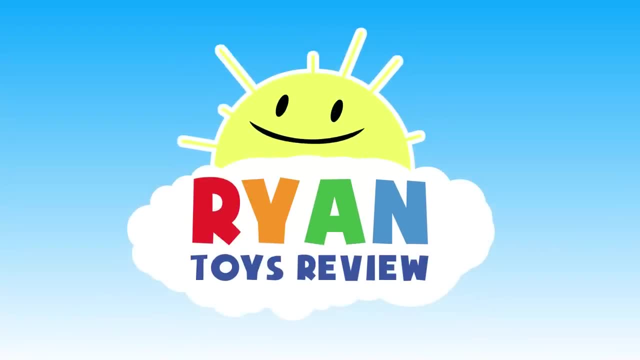 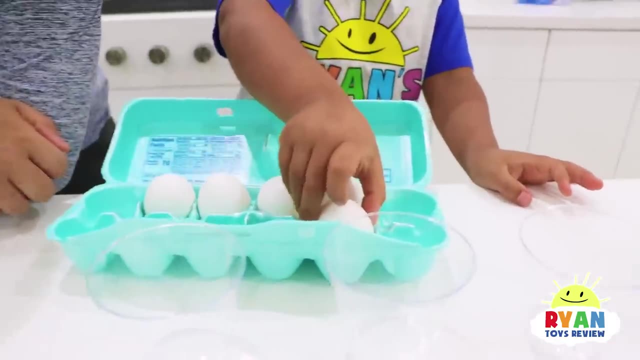 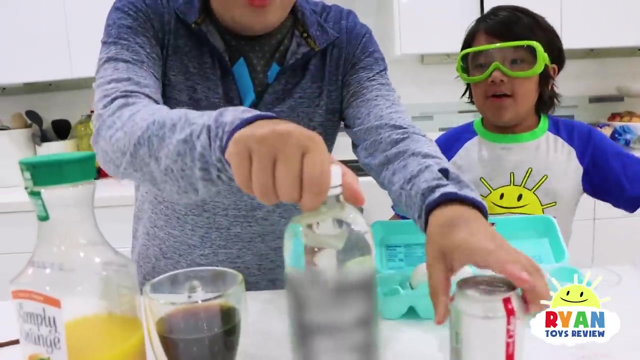 Welcome to Ryan's Toy Review. Hey guys, today we're going to do a science experiment and see what happens when we put these eggs in liquids. We prepared so many different kinds of liquids. We got Diet Coke, vinegar, coffee juice. 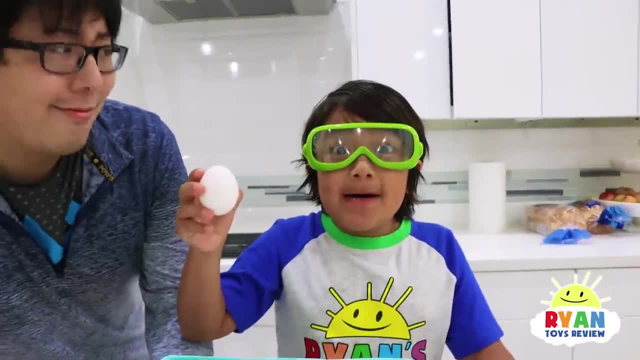 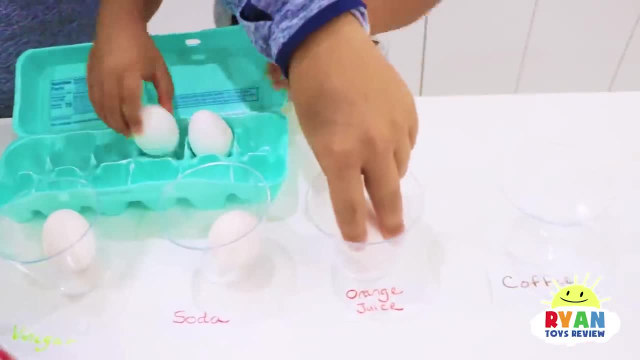 orange juice and water. Eggs are made up of a similar material as your teeth. We're going to put the eggs in each cup with the different liquids so we can test out and see what happens to the teeth if you don't brush it. 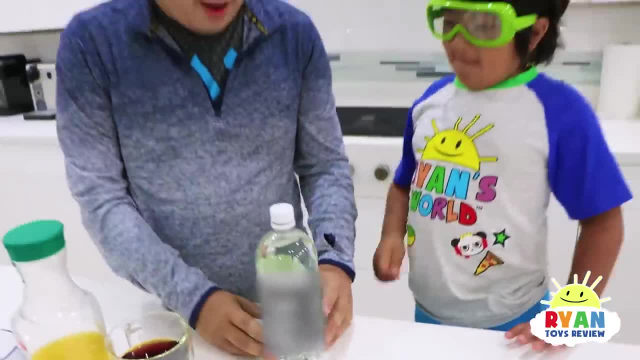 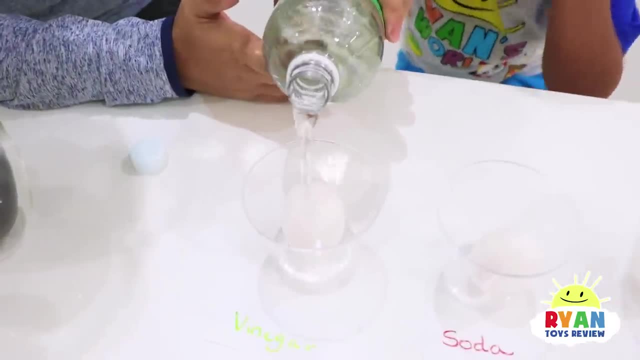 This one says vinegar. We're going to pour vinegar. Alright, here we go. Daddy's going to pour vinegar. Let's see, Oh yeah, it does smell like vinegar. Alright, perfect. Next is Coke. Pour this in too. 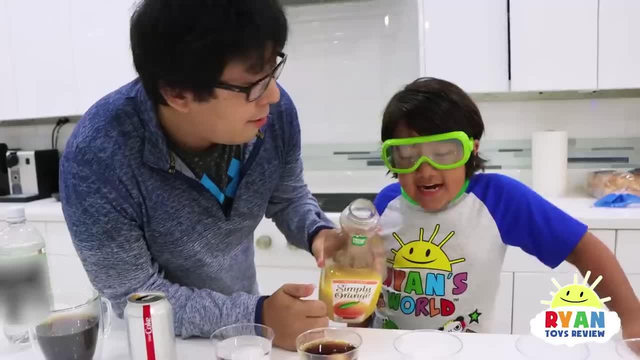 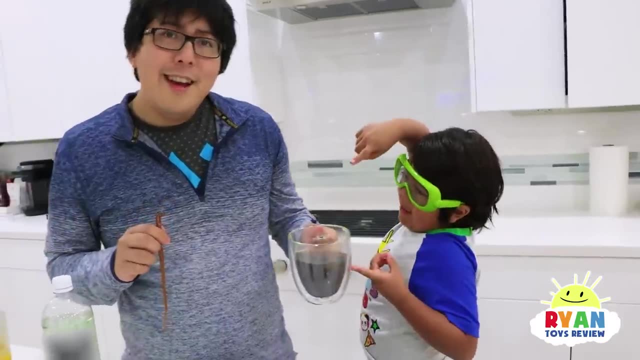 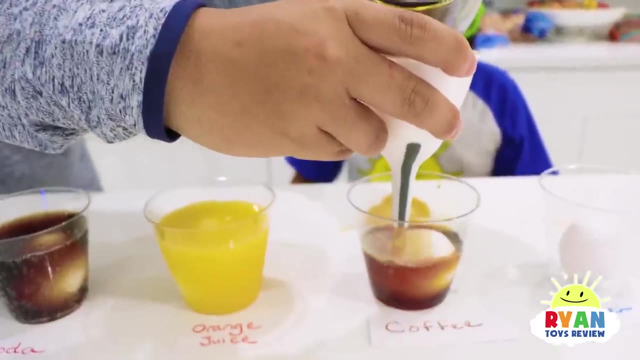 Ooooooooh, bubbly, Okay, all in. Next is orange juice. Ooooooooh, What's smelling. And the next one is coffee. Oh, oh, Next one is coffee. Alright, here we go. Ooooooooh. 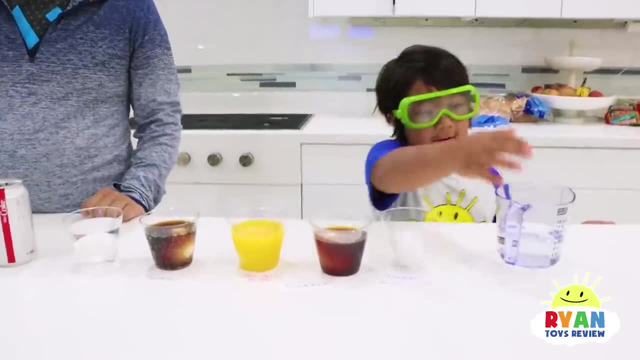 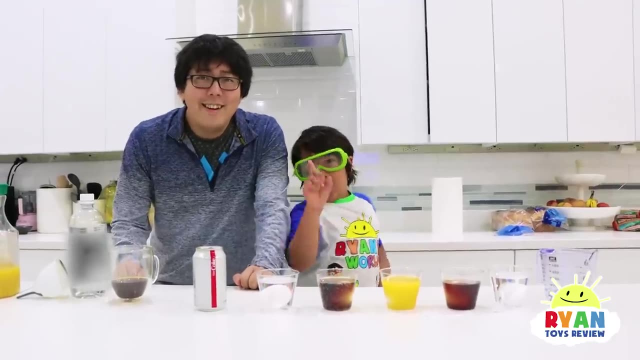 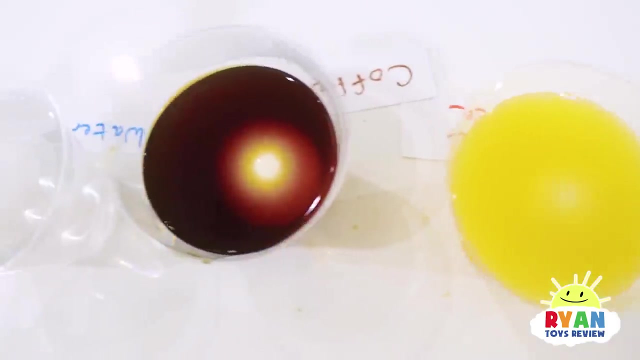 Coffee, Alright. Last is water Out of the way, and good job. Boom, boom. Now we're going to wait one day. See you soon. It's been one day now, and now we're going to check what happened to the eggs. 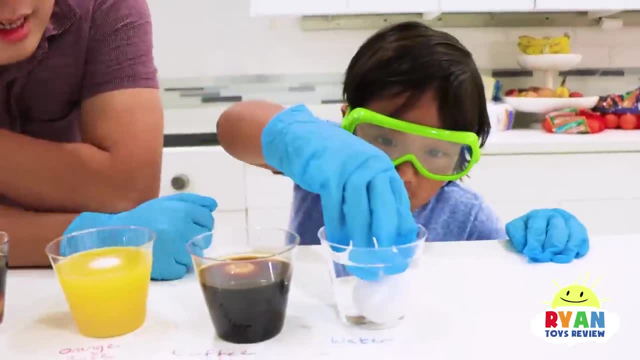 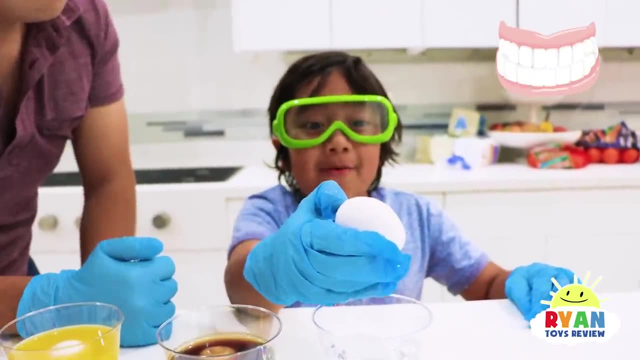 Now we're going to start out with water. Carefully touch it. Oh, it's the same. So the exact same. Yeah, nothing different, Yeah, so if you put your teeth in water for a day, nothing happens? Oh, okay. 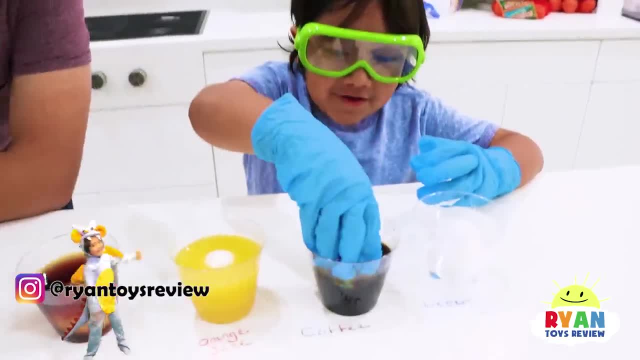 So water's good for you. Next, let's look at the egg in coffee. Oh yeah, I drink coffee all the time, so this is my teeth. Ahhhh, if I don't brush my teeth, Look at this. What happened to the egg Ryan? 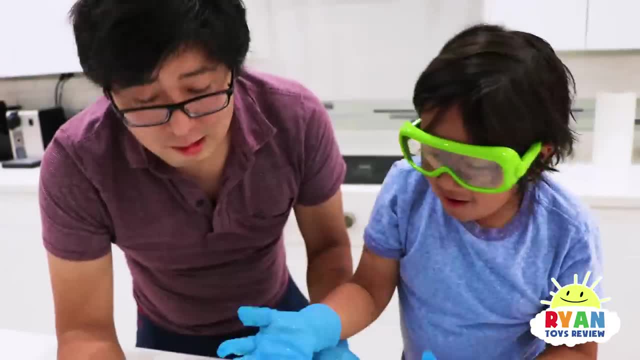 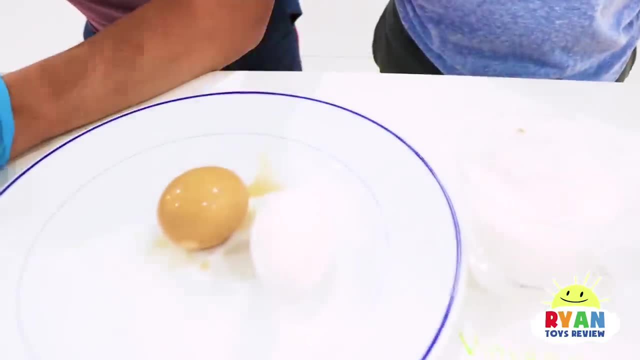 It's brown. It changed the color. look at it. So what happens? if you don't brush your teeth after you drink coffee? It's going to turn brown. I know no more white. This is what a normal egg looks like. 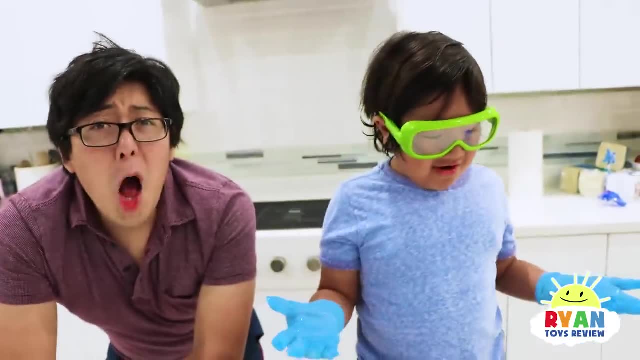 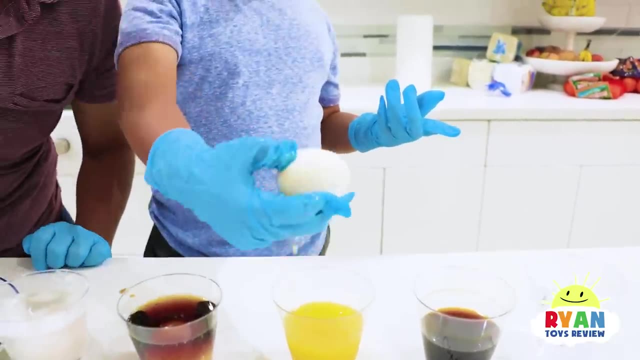 and this is what an egg in coffee looks like. Ewww, Noooo. Now let's try orange juice. It can't be orange, right Color? Let me see What. Oh, you see the bubbles that are on it. 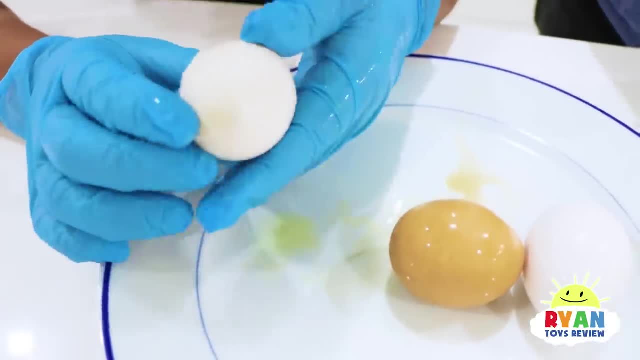 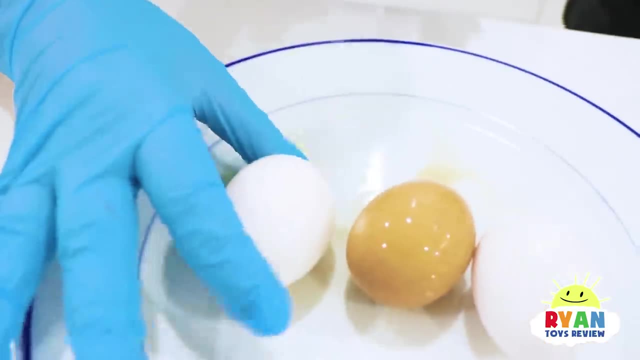 Yeah, but besides that, it's the same right. Don't forget, there's sugar on there too, so if you leave it for a while, it might attract bacteria and germs. Ewww, I'm going to stop touching that. 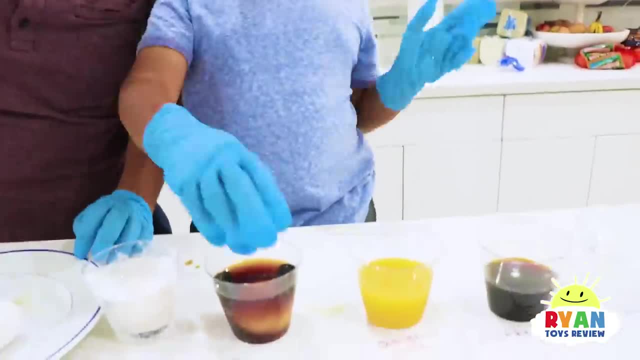 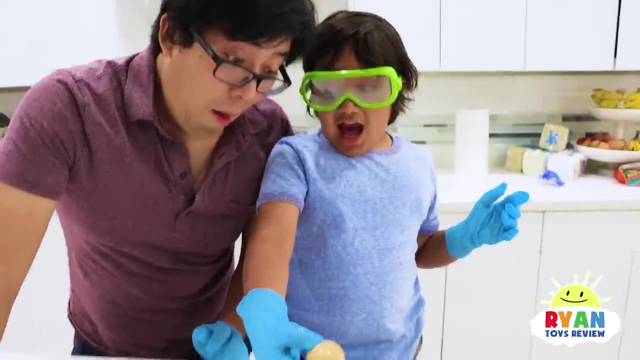 Now we're going to try soda or Coke. Oh yeah, we hear all the stories about soda. Let's see what happens. Yeah, and soda also has lots and lots of sugar. What Ewww? Oh no, it also stains the egg. 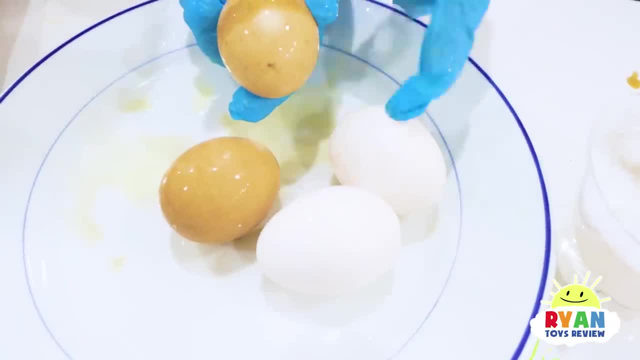 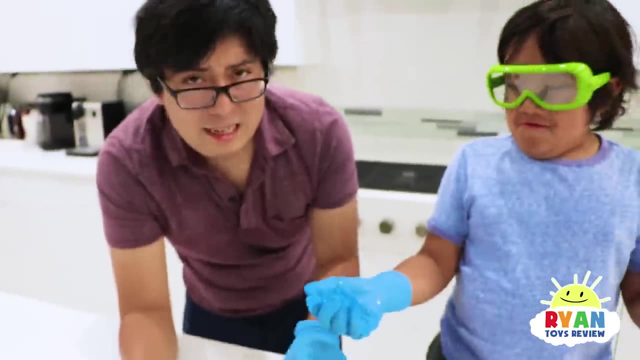 Wow, Wait. so this is like a super good version. This is a second best version. This is the worst version. No more white teeth, right, Yikes? This is the most exciting one, Vinegar. All right, let's see. 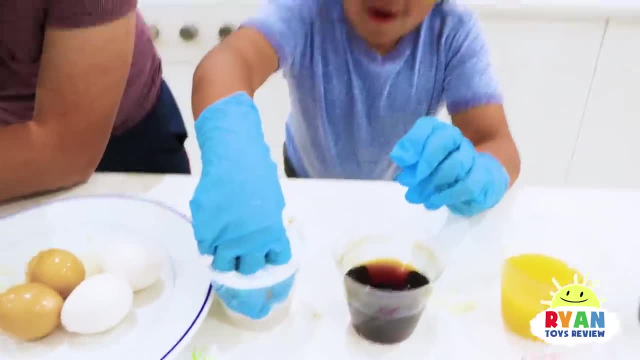 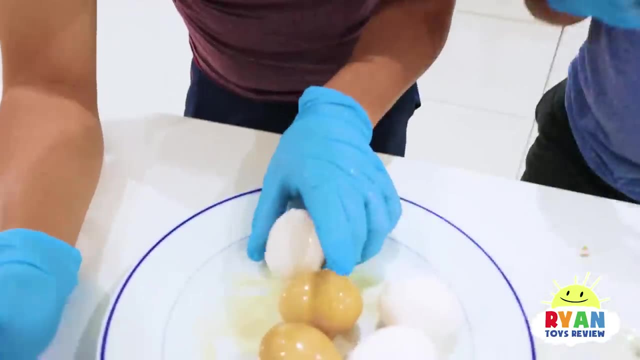 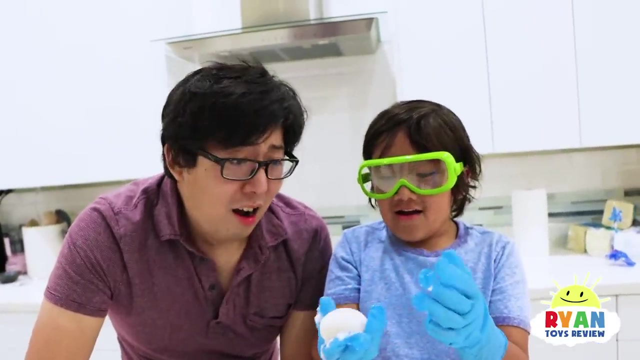 Take it out, Ryan. Take it away What You got to be gentle. What happened? Feel it. feel it. Oh, it's soft. What happened? What happened to the shell? Vinegar is very acidic, so it actually dissolves the shell. 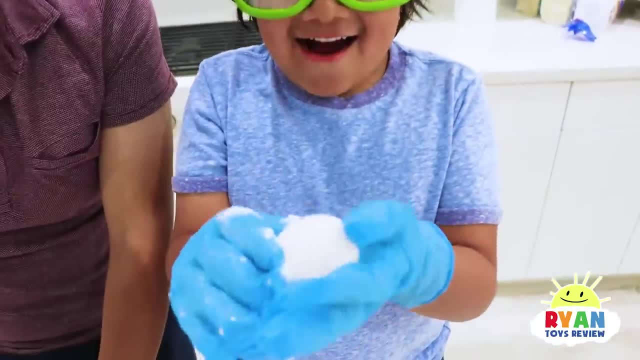 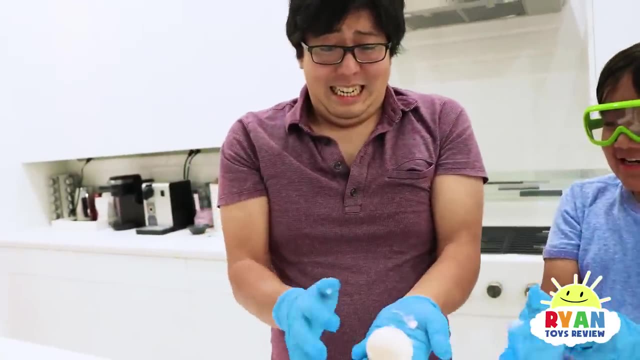 The shell is gone. Ryan, I knew it. It's all you left. Oh, those squeeze-like eggs. It's going to explode. It's like a bouncy egg You dare to bounce? Yeah, They don't Huh. 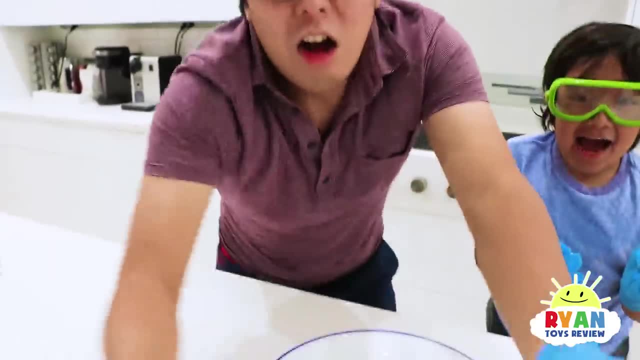 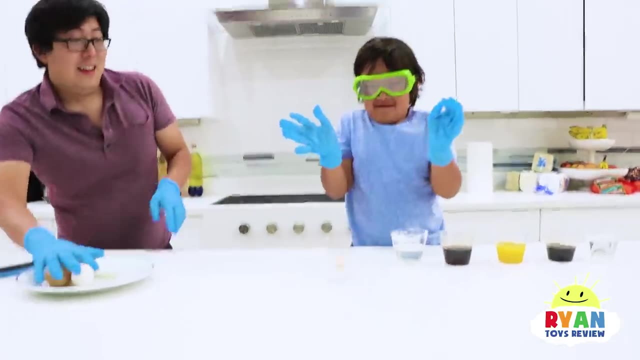 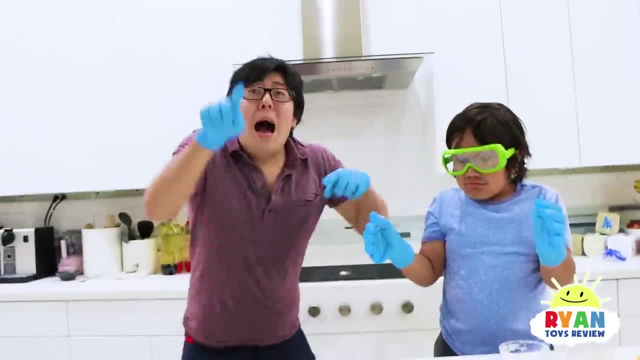 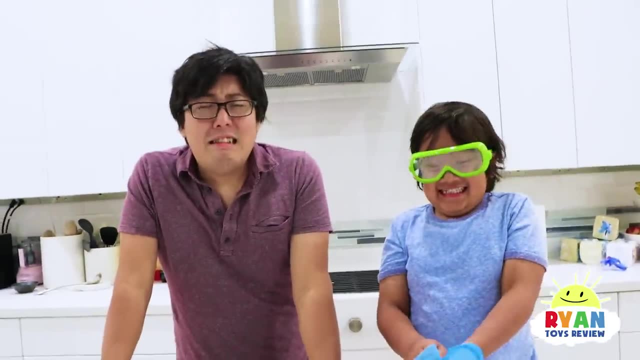 Ah, Ah, Ah. Ah, Mommy, you lied, So maybe we should have kept it in there a little bit longer. It'll only be a day, so maybe you need two eggs. So there it is, the shell there. 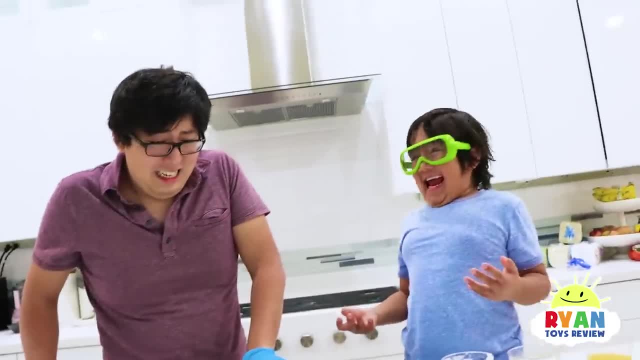 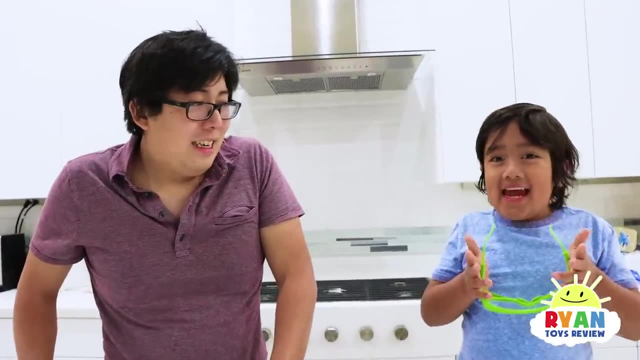 So Ryan probably bounced it a little bit too much, but if you leave it in for two days it's actually more bouncy, Wow. So now you know what happens to vinegar. What does it do? It dissolves, Dissolves. 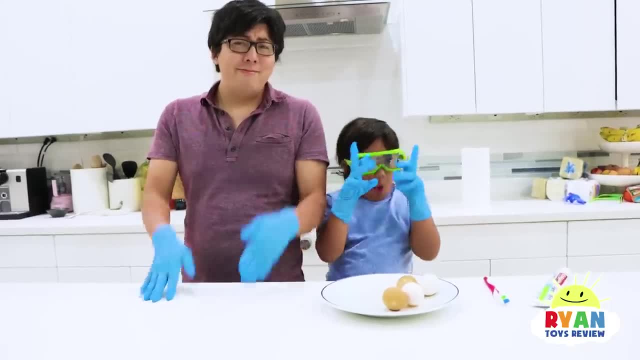 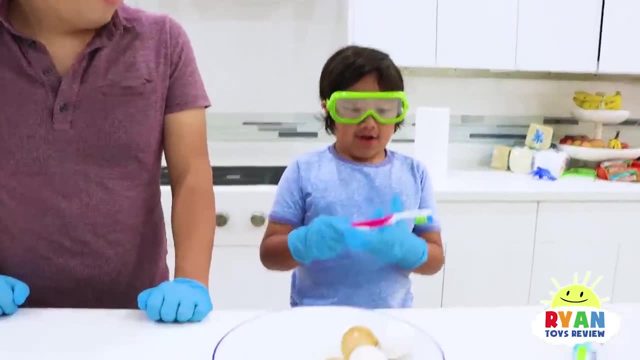 All right, guys, Clean up time, We're back. We cleaned up, We got new gloves, right. And then Ryan learned not to touch raw eggs, right, Yeah, Ryan, also go wash his hand already. So now do you see how the eggs that was in coffee and soda was brown? 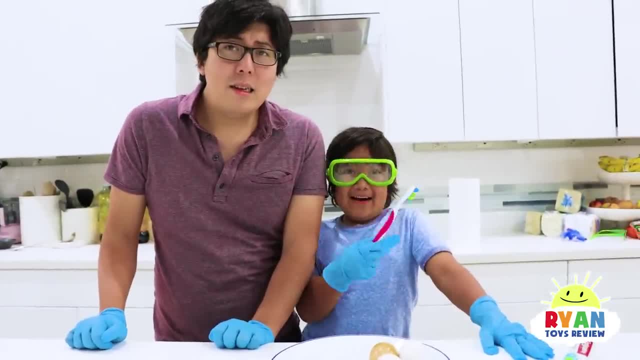 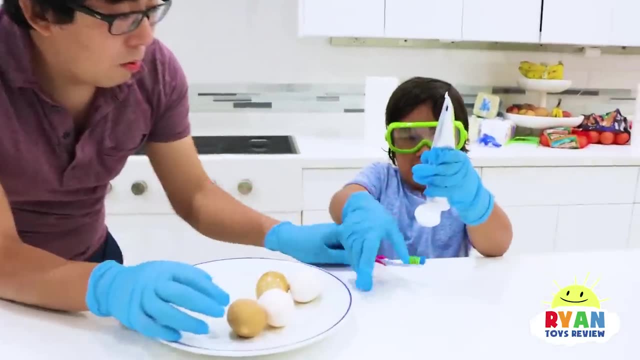 Mm, We're going to test it out, to brush it, Yeah, To see if it has any effects. Okay, Yeah, All right, Yeah, Make sure you put the toothpaste on. Oh, Be careful, Teamwork Ugh. 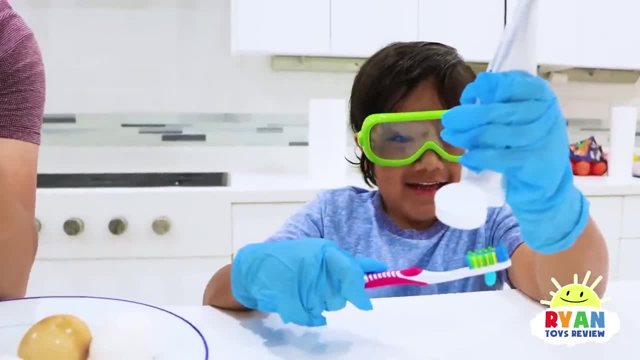 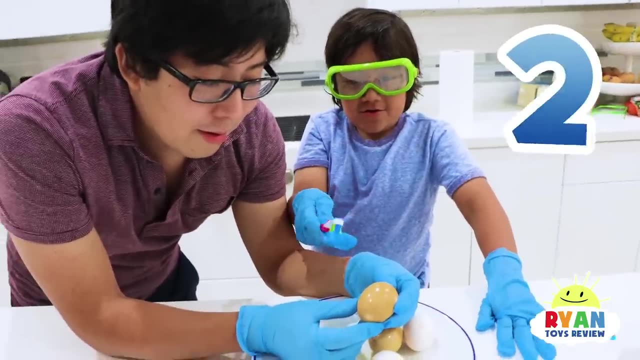 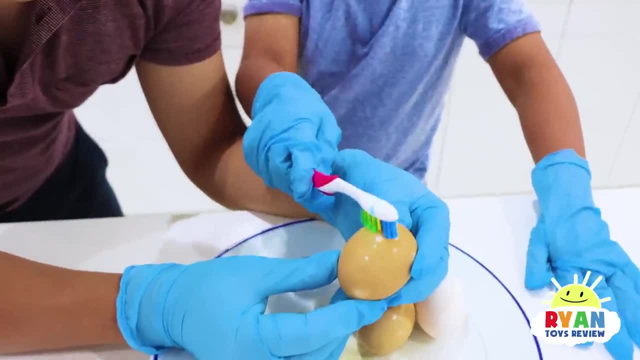 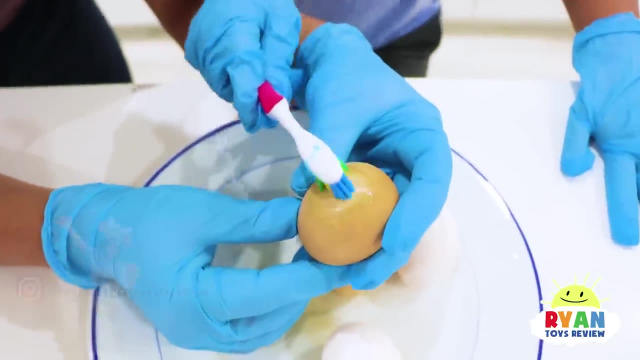 Brushy, brushy, brushy. Ten hours later, No, We're seeing if it works. Whoa, Whoa. I can tell already: Does brushing help make your teeth whiter? It does. Oh yeah, I see it. 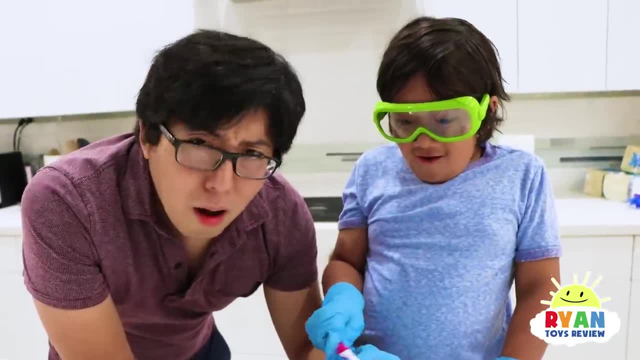 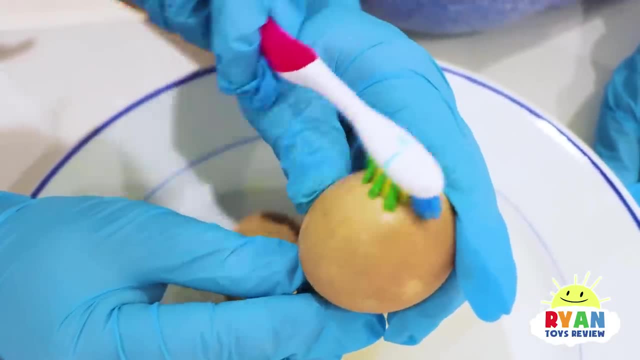 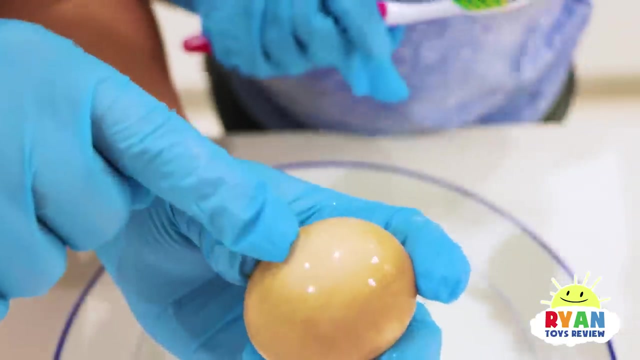 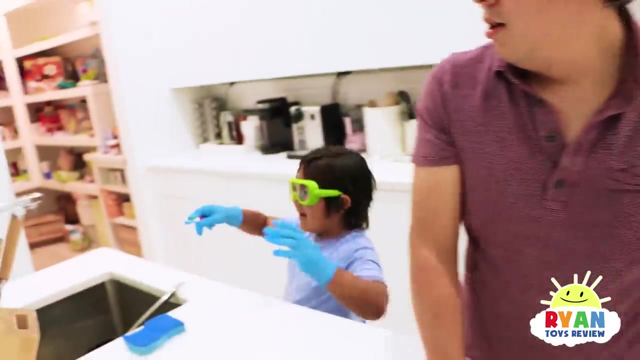 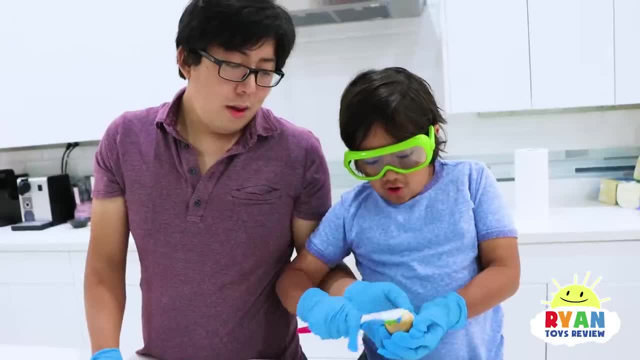 You guys see, Oh, look at it, It's already the difference. This is the regular spot and this is where we brushed it. Oh yeah, Look at the color. Yeah, Wow, The importance of brushing your teeth, right? 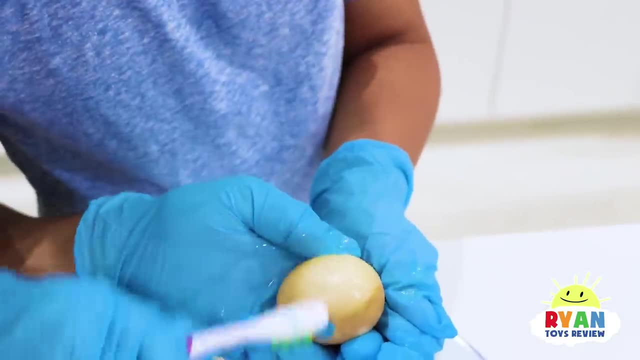 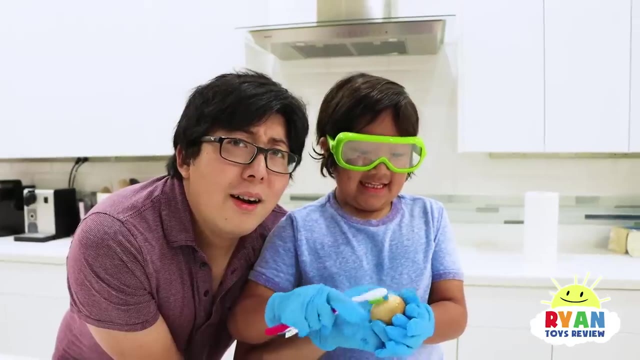 Mm-hmm. Do you see the difference? Yeah, I can tell It's nice Big difference. So what did you learn, Ryan? That brushing your teeth helps a lot. Yeah, it does. And how many times a day you're supposed to brush your teeth at least? 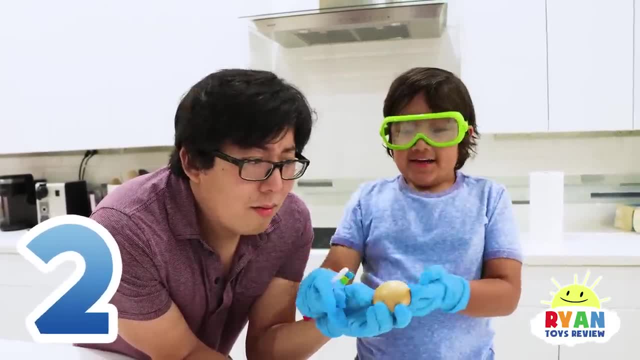 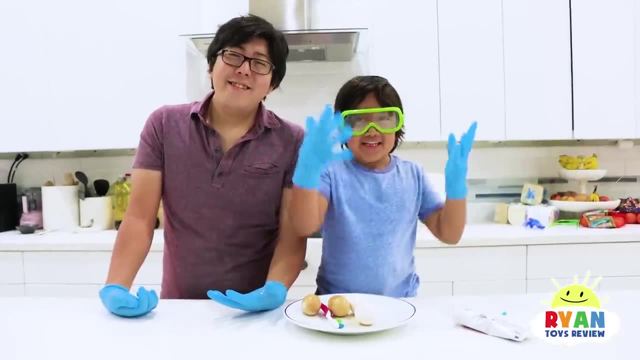 Two, Two times a day. Good For how long Do you know? Two minutes, Two minutes- Yeah, Easy to remember. Thank you for watching. I hope you like this science experiment. Bye, Bye, Remember. always stay happy and rise up.